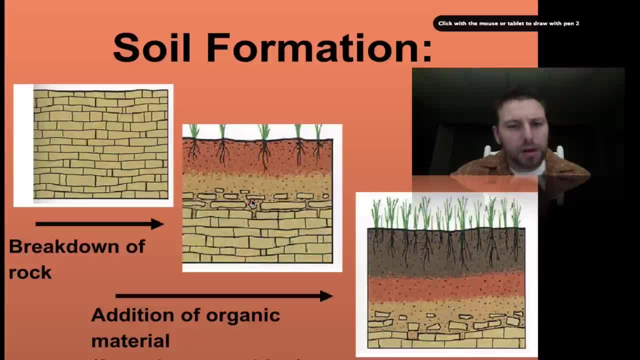 weathering processes will break down, and we can see that right here. As it breaks down, the sediments pile up. so we can see: here there's a pileup of sediments and ultimately, what's going to happen is that, as these sediments are going to pile up, we have organic material also. 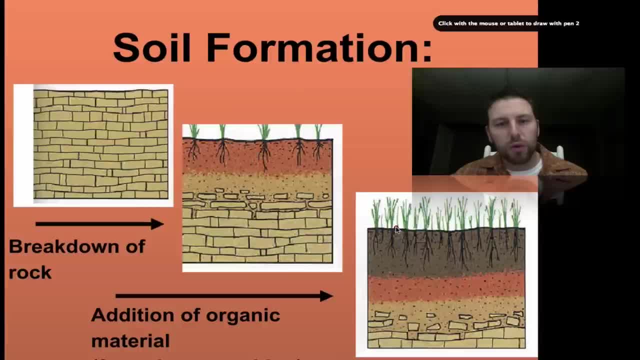 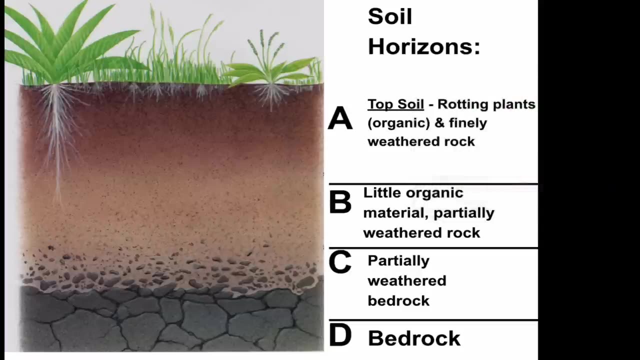 up on top or plants growing. As the plants grow and possibly die, they'll contribute more organic material to the top. The organic in this situation here is once living organisms. We have a number of different soil horizons or soil layers. We have the O up on top, which is 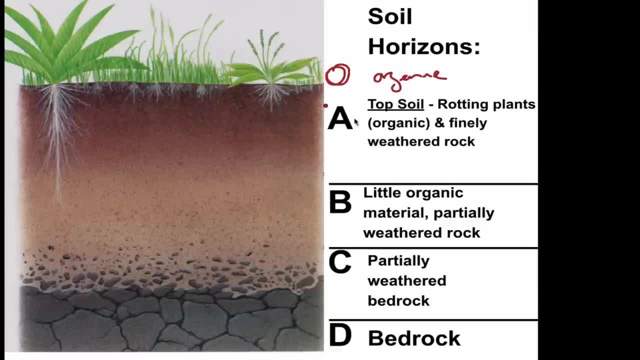 our organic layer containing all of our plants right here. Then we have A, our topsoil, and you can see that as we go down, the colors change a little bit. So this region right here is our topsoil. from here to here, Rotting plants, organic and finely weathered rock, We have a. 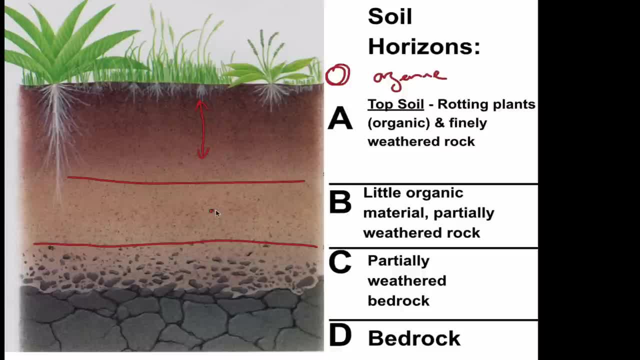 B horizon and you can see here it's mostly the same color- Little organic material right We're farther away from it- Partially weathered rock in this region. As we get to the C or the regolith we can see that it's some bedrock broken down into bigger pieces. 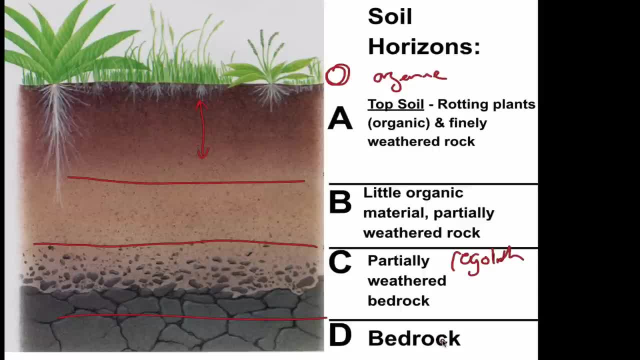 and then finally, a D horizon, which is bedrock, right here. Sometimes you'll have all these layers, sometimes none. It depends on the area, but in a typical region where we have the breakdown of bedrock and with given enough time and little disturbance, we'll get the 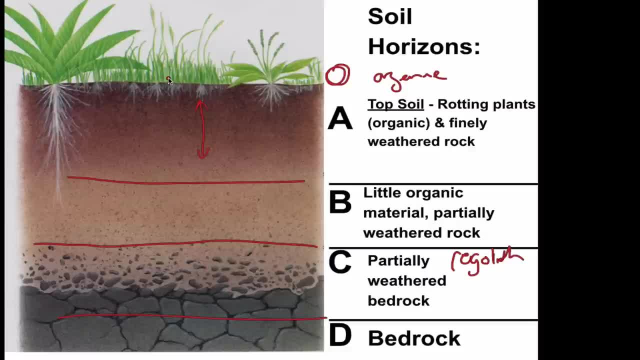 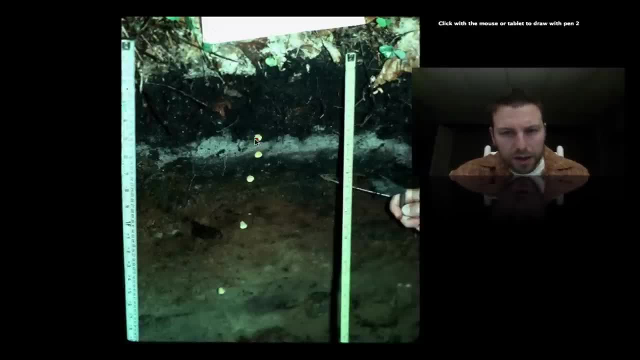 sediments to pile up with organic material up on top Here this person made a cross section and these and marked the different horizons. So you can see here with these little T's they mark the number of different soil layers that we have in here. Okay, yeah, that's pretty. 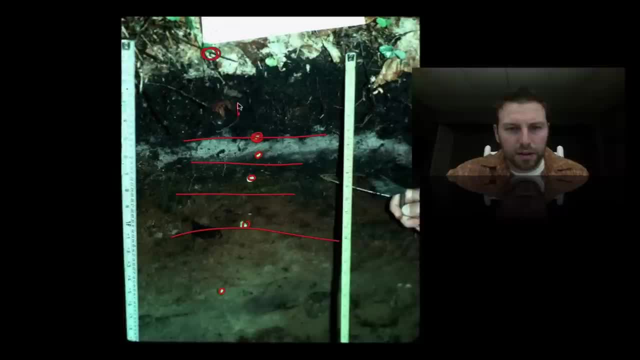 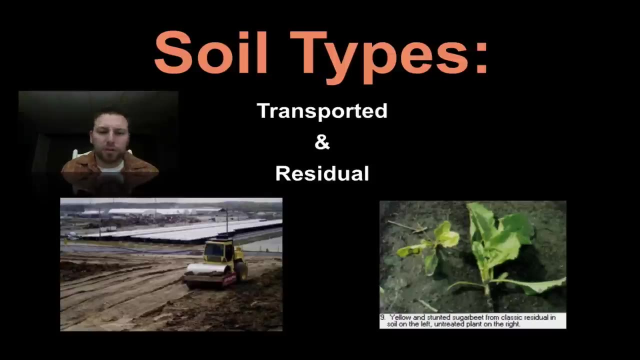 easy to see as we get to the top. So we have our organic layer right here, A for topsoil, B, C and I think the D is way down here. They're probably a couple layers off, but there's definitely distinguished differences between these Soil types. There are two major types of soil. We